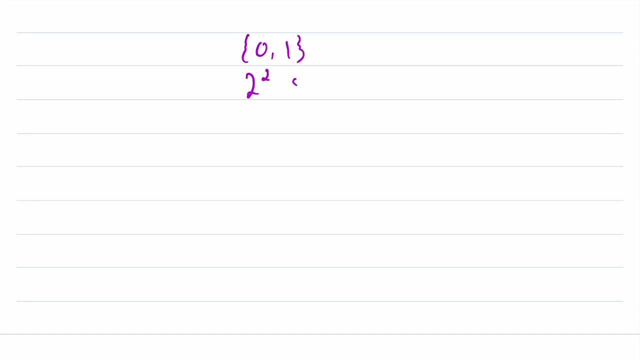 this set, So it has two to the power of two subsets and two to the power of two. that's two times two, which is equal to four. So this set has four subsets. And since it only has four subsets, let's go ahead and write those subsets down. The empty set is a subset of every. 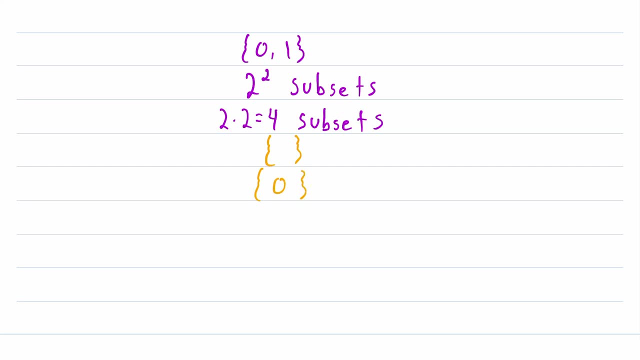 set. Then we also have the set containing zero, that's a subset, And the set containing one, that's another subset. And then the last subset is the set containing zero and one. this set has two elements. therefore it has four subsets, And here those subsets are. 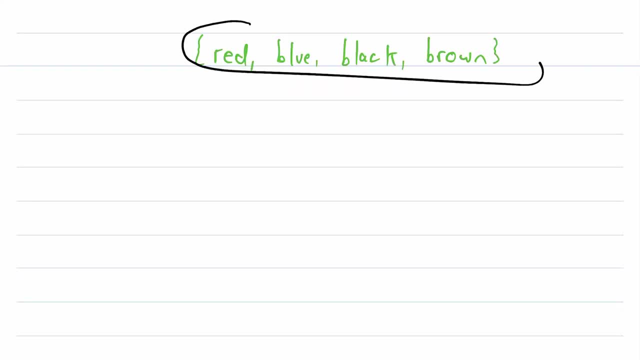 Alright, let's move on to another example. How many subsets does this set have? Well, how many elements does it have? The elements are separated by commas, so we can pretty easily identify those: 1, 2,, 3, 4.. This set has 4 elements, Thus it has 2 to the. 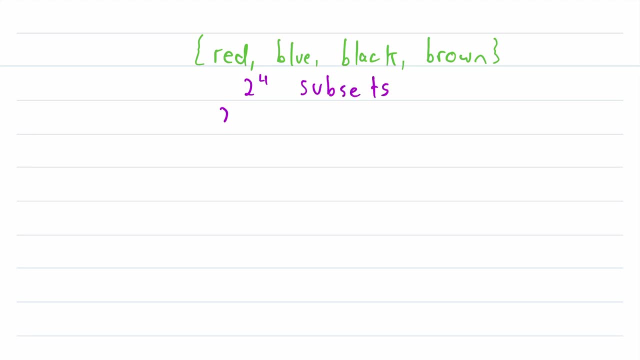 power of 4 subsets. So that's 2 times 2 times 2 times 2, which is equal to 16.. 16 total subsets. Again, to find the number of subsets that a set has, all you need to do is raise 2 to the power. 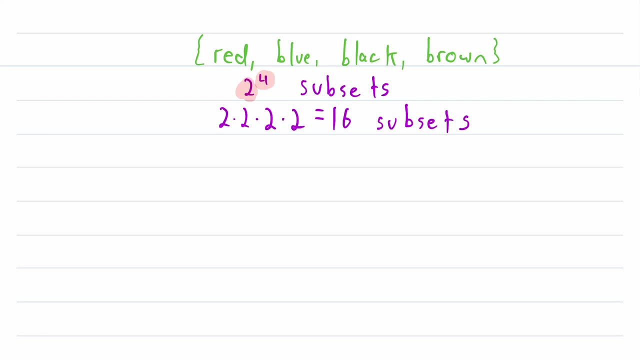 of the cardinality of the set. Remember that the cardinality of a set is just the number of elements that it has. So this set has 4 elements, so it has 2 to the power of 4, 2 to the power of. 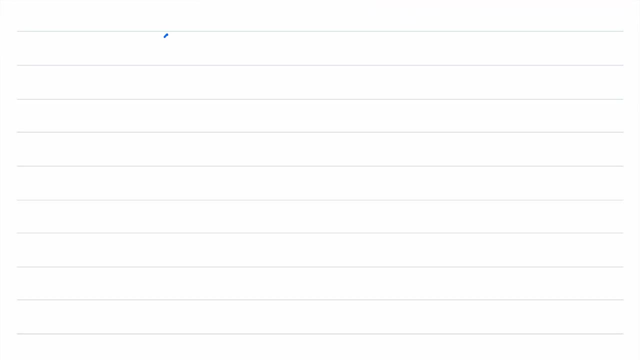 4 subsets. All right, let's do another example. This will be our last one and I'll just try to make it a little bit trickier than the others. All right, so here's a bit of an example: Ugly set: How many subsets does this set have? Of course, we need to figure out how many elements. 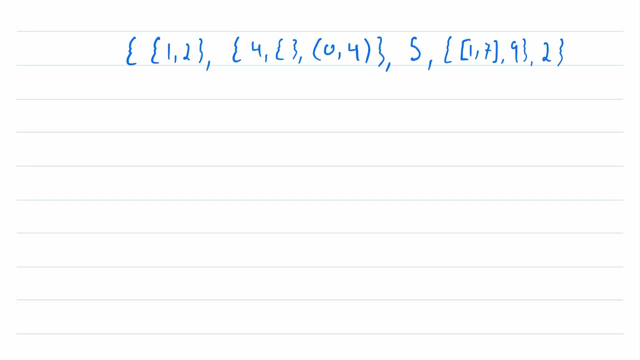 it has. I just did a video on how to identify the elements of a set when it's kind of a nasty set like this, So I'll try to leave a link to that video in the description too. Check that out if you're not sure how to identify the elements in a set like this Using the strategies that I discuss. 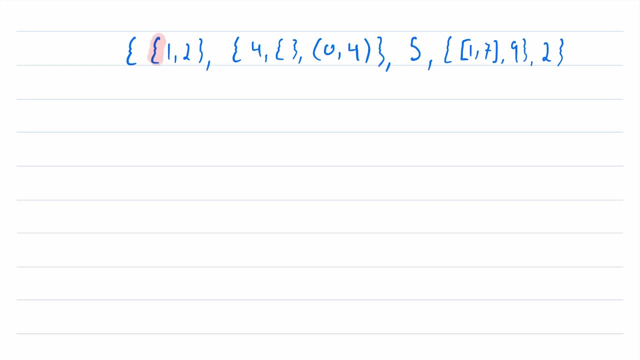 in that lesson we can see that one element starts here and then it stops when this bracket is closed. So that's one element. Then we see another element starts here and it stops when that curly bracket is closed. That's a second element. Then we have a third element and a fourth element starts at that curly bracket. 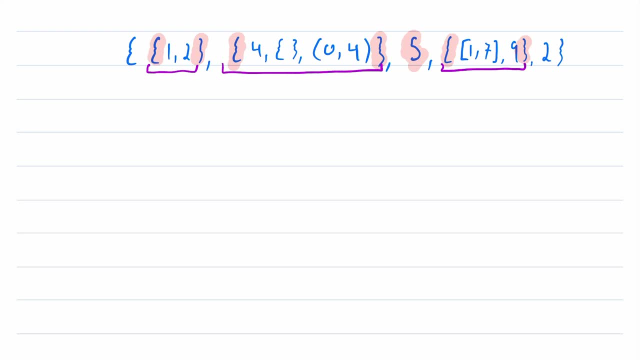 which gets closed there. So that's the end of that element. And then we have one more element right there. Let me underline the 5 and the 2.. So we've got 1, 2, 3, 4, 5 total elements, And again. 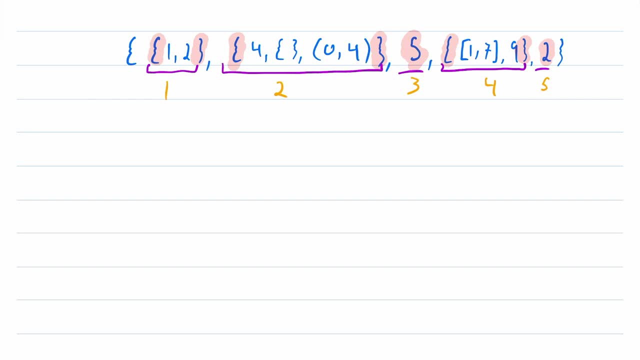 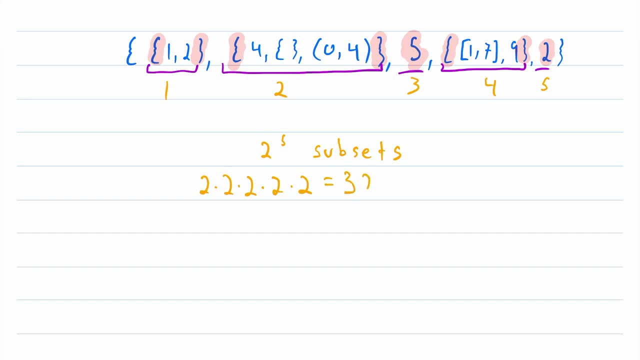 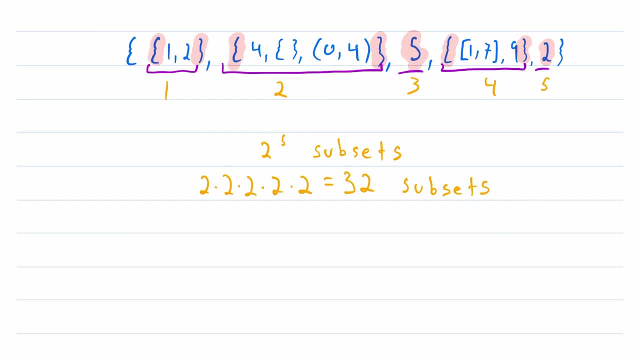 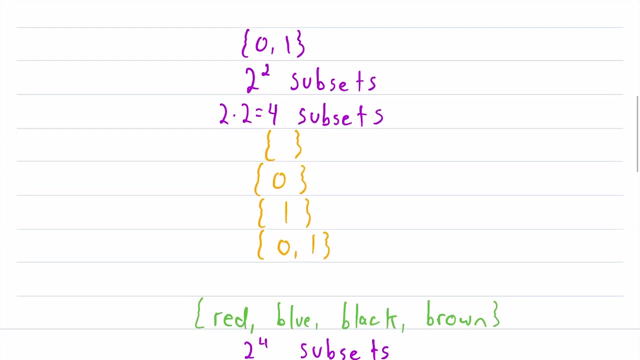 all there is To it. to figure out how many subsets a certain set has, all you have to do is raise two to the power of that sets cardinality. So if it has five elements, then it has two to the power of five subsets. If it has four elements or, excuse me, two elements. looking at this first example, 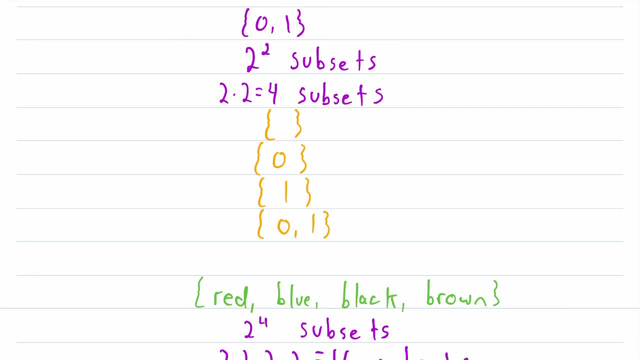 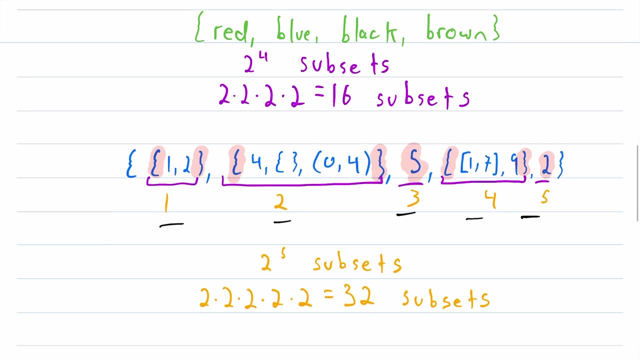 if it has two elements, then it has two to the power of two subsets. And if it has four elements, then it has two to the power of four subsets. And with all that said, I'll just leave you with a couple of practice problems to try on your own. 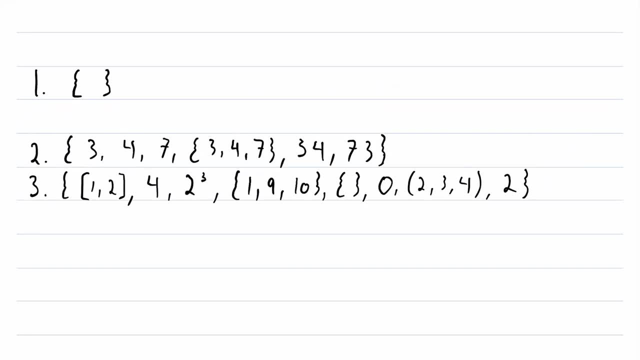 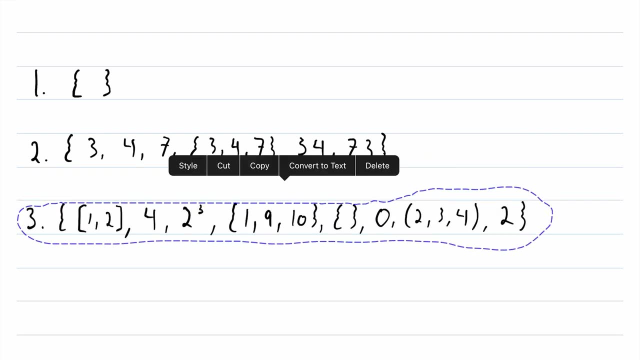 Alright. so here are a few nasty examples, three of them to be exact. try to figure out how many elements are in each of these sets And then, from that information, figure out how many subsets each set has. Let me know what you get down in the comments And I'll leave the solutions in the 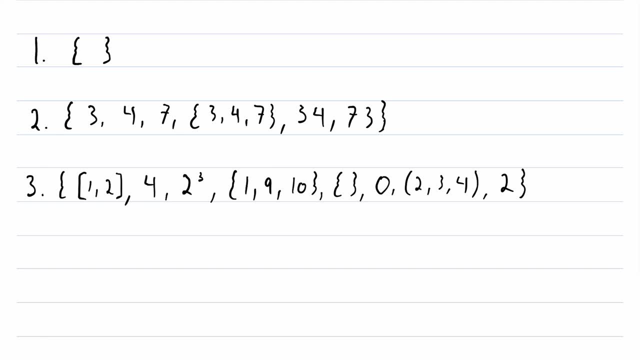 description. Thank you very much for watching. Let me know in the comments if you have any questions, need anything clarified or have any other video requests. I'll see you next time and be sure to subscribe for the swankiest math lessons on the internet. And a big thanks to Valo who, upon my 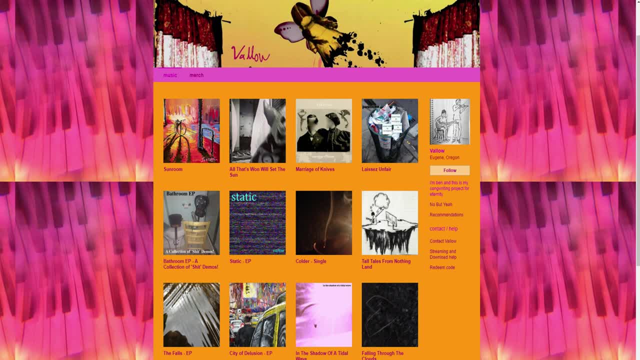 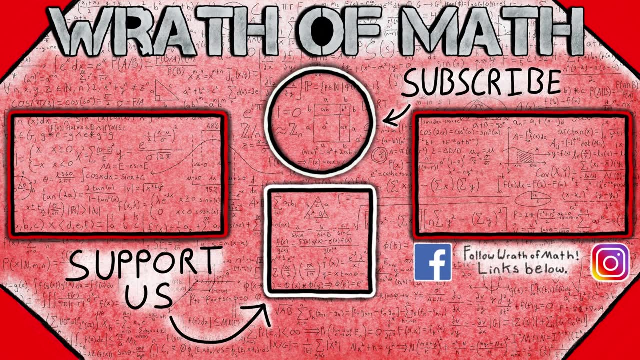 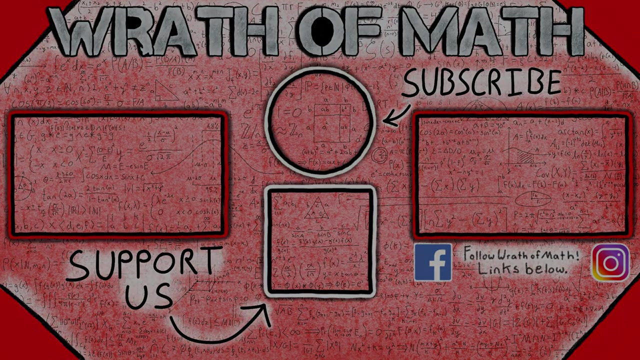 request: kindly gave me permission to use his music in my math lessons. Link to his music in the description. It's not cool.